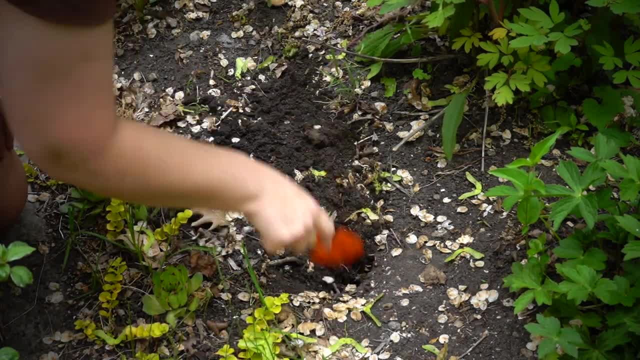 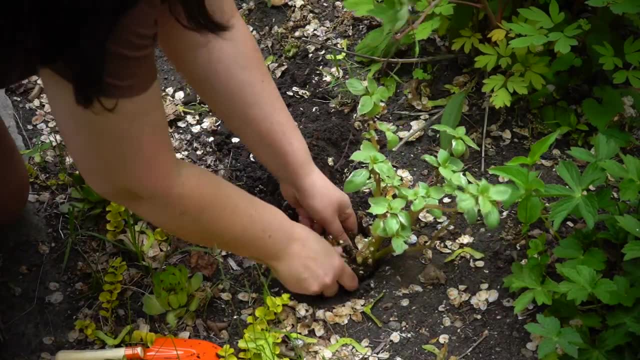 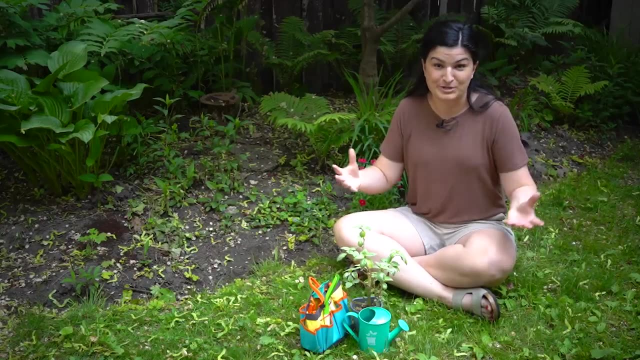 look for plants that are a little bit more robust, because if the child is given the responsibility of watering the garden, there's a very good chance that this plant, this area of the garden, is going to receive quite a bit of water. So look for plants that will be okay being overly. 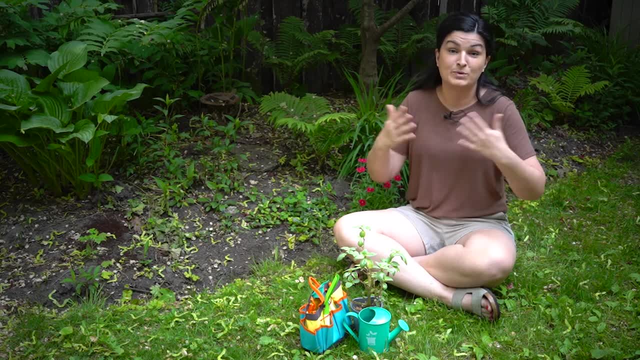 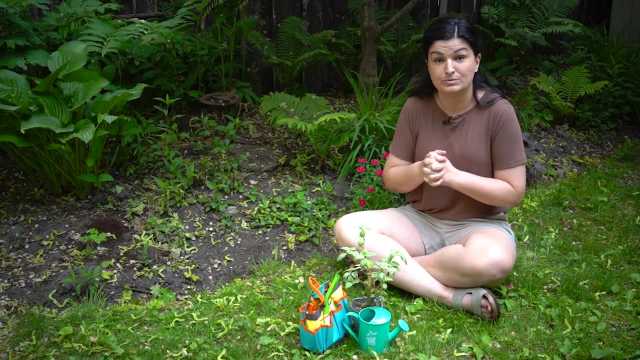 watered. I can tell you from experience in the classroom, our plants were never thirsty. So if you're looking for some ideas, we do have them in a blog post that I will link to in the description below. So yes, with things like watering the garden, you can give them access to the hose, or you. 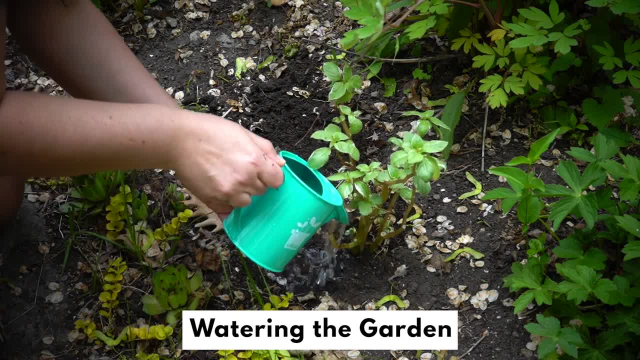 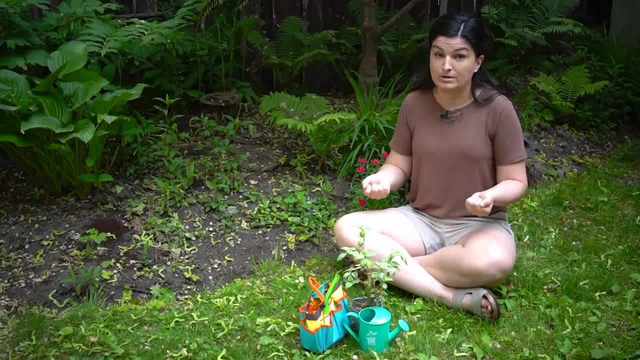 can just have them water the garden. So if you're looking for a plant that's going to be a little bit more robust, just have a little child-sized watering can and show them how to water the garden, test the soil to see if it's dry, and so on. A wheelbarrow is a wonderful gardening tool for. 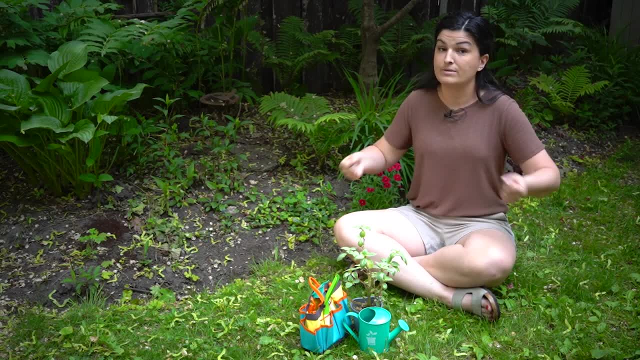 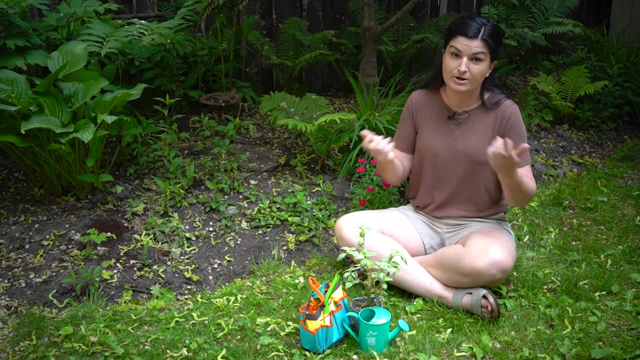 children around the age of two and three. It's another really great maximum effort activity. You just put some soil in there and they can move it around the garden, dump it in the garden and so on. And then, lastly, if you do have the space, 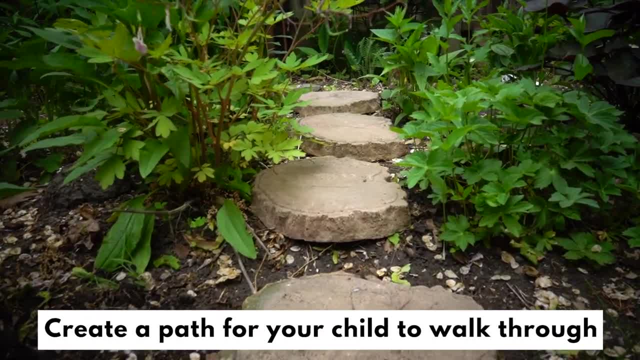 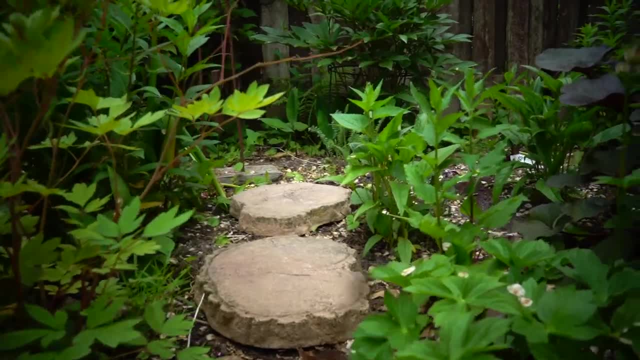 it's really nice when planning out your garden if you could sort of create a path for your child to be able to walk through. That way they can really sort of immerse themselves in the garden. They can walk around, explore, see everything that the garden has to offer. 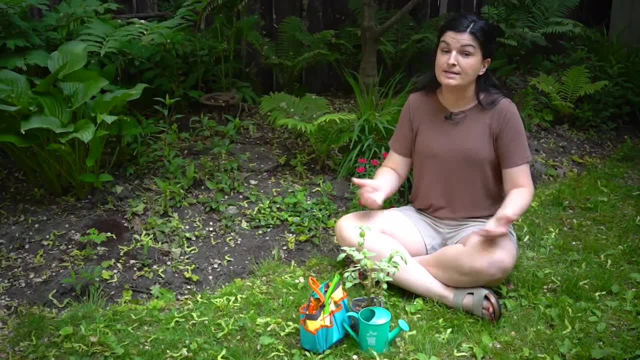 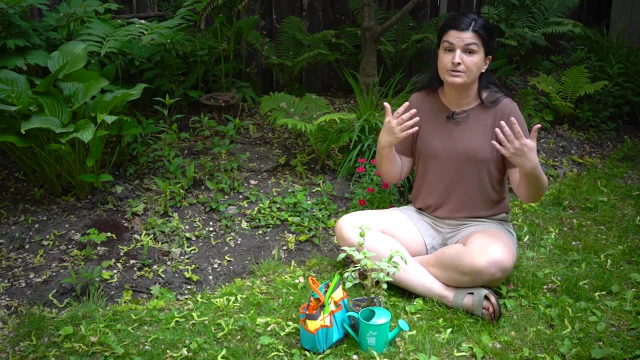 and learn so much about nature while doing it. So if you're interested in learning some more about the developmental benefits of gardening, I mentioned a blog post earlier. I'll link to it in the description below, but it's called Six Montessori Gardening Activities for Infants. 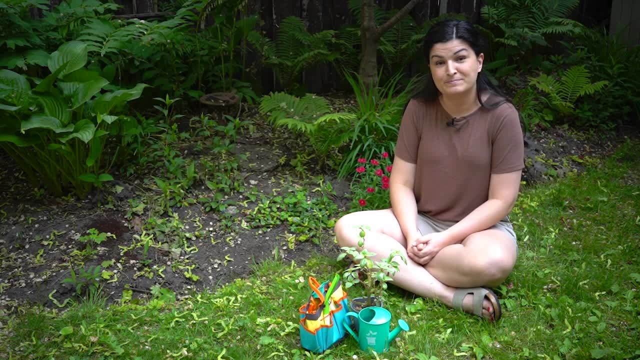 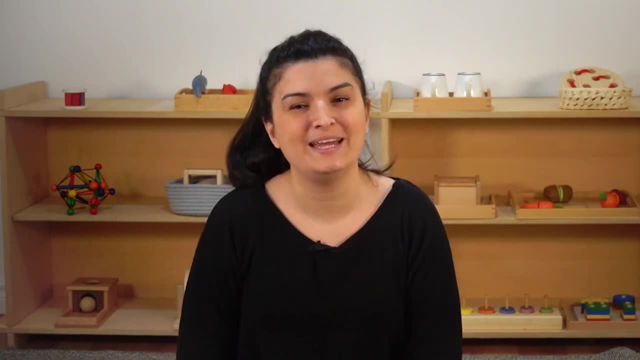 and Children, and you'll find some more information there. So I hope you enjoy and I'll see you next time. Bye, Thanks for watching. If you liked this video. it really helps our channel if you like and subscribe. This helps other parents to find. 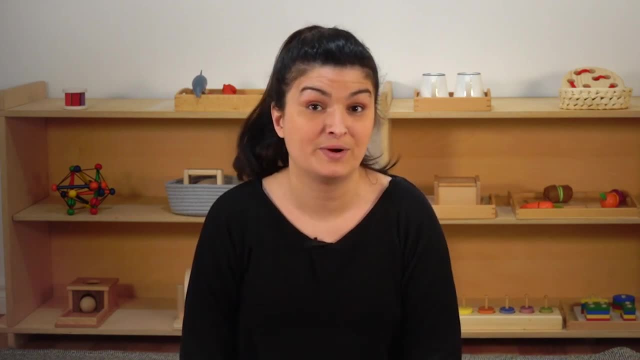 our channel And if you have a question, feel free to comment your question below and we'll answer it in a future video. Take care, Bye.